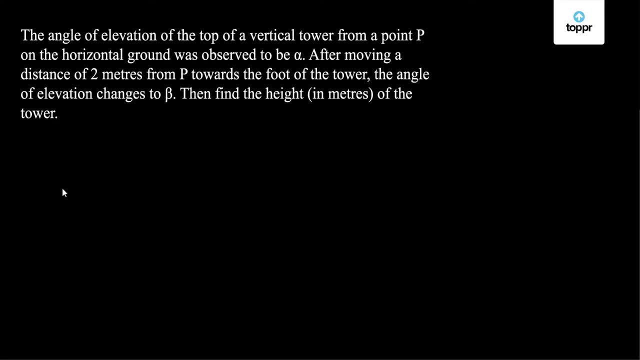 So let us see one problem based on trigonometry. This problem had appeared in JE Main's examination in 2014.. The problem is: the angle of elevation of the top of a vertical tower from a point P on the horizontal ground was observed to be alpha. After moving a distance of 2 meters from P towards the foot of the tower, the angle of elevation changes to beta. Then find the height in meters of the tower. So we will try to picture as what has been given to us. 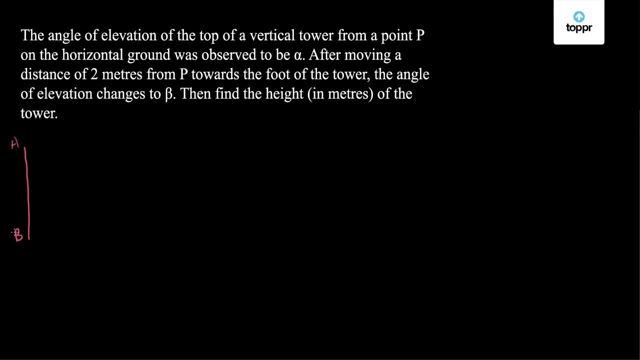 So I have a tower here, Let's say AB, of height H, and I have a point P on the horizontal ground and the angle of elevation here is alpha. And as I move towards the foot of the tower, that is, towards point B, I reach a point C. So I have covered 2 meters and the angle of elevation here changes to beta. So with this information I have 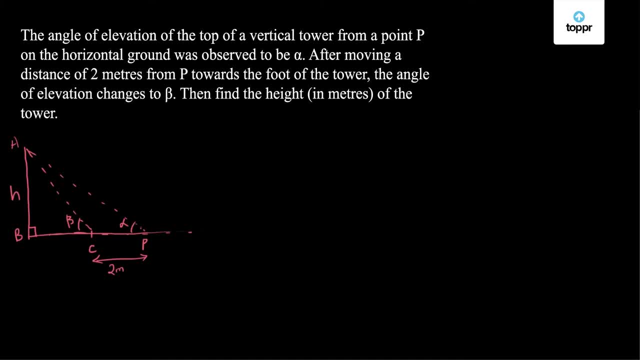 to find the height H of the tower in meters. So in right triangle, ABP- I have tan of alpha- is given by H upon BP, which means BP is equal to H by tan alpha. Similarly, in right triangle, ABC I have tan beta is equal to H upon BC. So I have BC is equal to H upon tan beta. I know that BP minus BC is 2 meters. 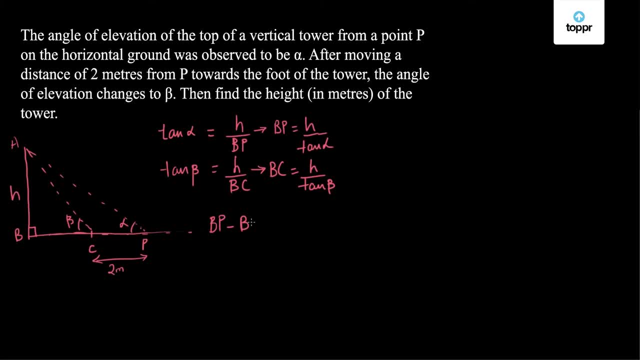 So I will make use of this fact. BP minus BC is equal to- and I will take the values from here- So I have H1 upon tan alpha minus 1 upon tan beta. 2 is equal to H times tan beta minus tan alpha upon tan alpha tan beta. So I have: H is equal to 2 times tan alpha tan beta upon tan. 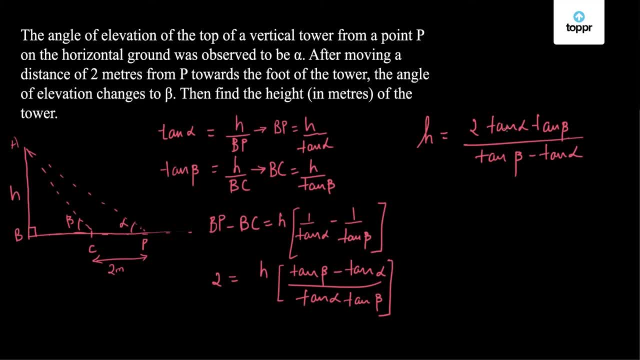 beta minus tan alpha. To simplify further, we will write tan alpha as sin alpha by cos alpha and tan beta as sin beta by cos beta. So we will end up with 2 sin alpha, sin beta upon sin beta, cos alpha minus cos alpha, cos beta, sin alpha. So this is the expansion for sin of beta minus.